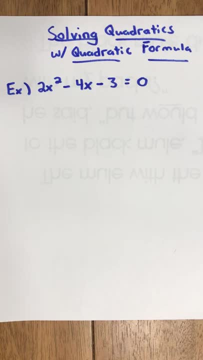 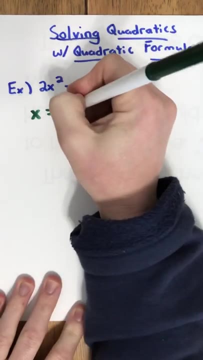 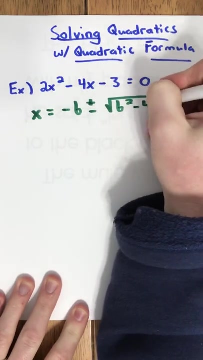 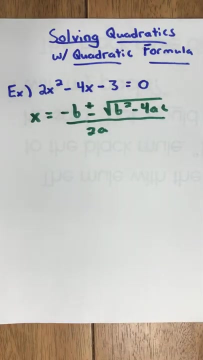 happen in particular inside that square root towards the end. Alright, so we're going to write out our quadratic formula: x equals negative b plus or minus the square root of b squared minus b all divided by 2a. And just a reminder from the last couple days, when we have a quadratic, 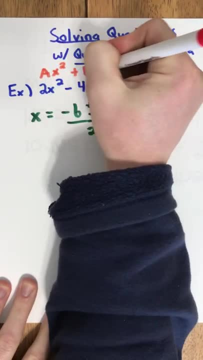 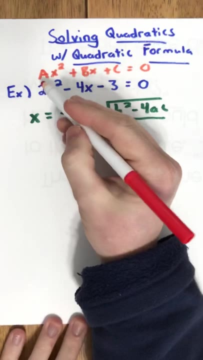 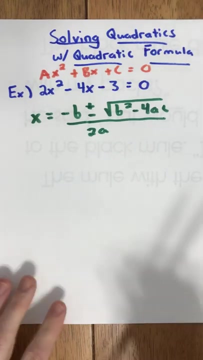 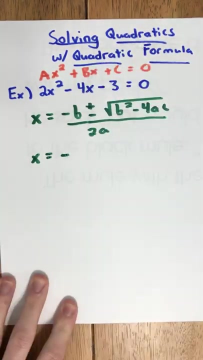 we're talking about ax squared plus bx plus c. So hopefully you can clearly see here: a, in this case, is 2, b is negative 4, and c is negative 3.. So we're going to go ahead and plug that in. So we're going to have x equals negative b, Now b is negative 4, so negative, negative 4. 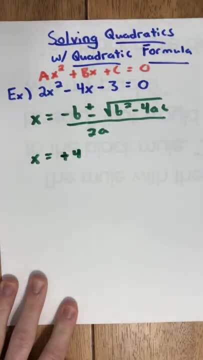 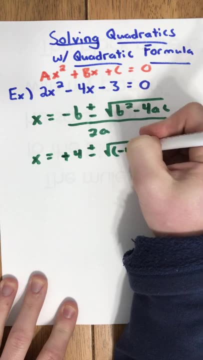 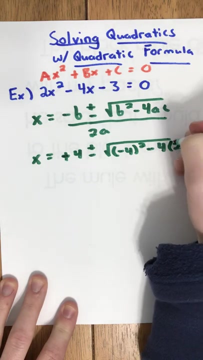 is going to make this a positive 4, the opposite of negative 4, plus or minus the square root. b is negative 4 squared minus 4.. a is going to be 2 here and c is going to be negative 3.. 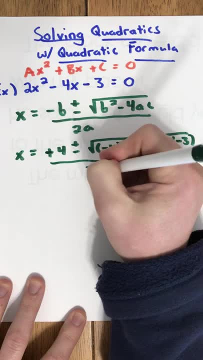 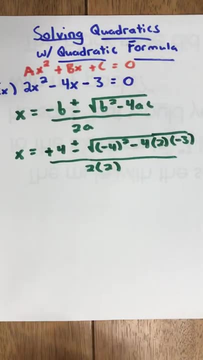 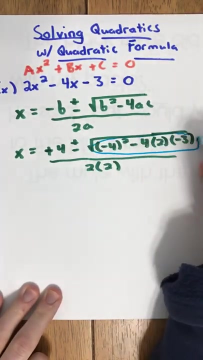 And we're going to divide that by 2a, which is 2.. Alright, so again, just like the last couple days, I'm going to advise that you start to simplify this by taking care of what's inside this square root. initially, Be careful when you're putting this in your calculator. make sure that you put 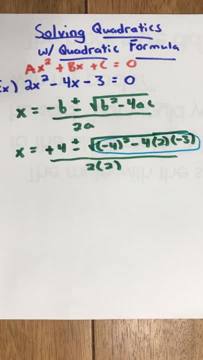 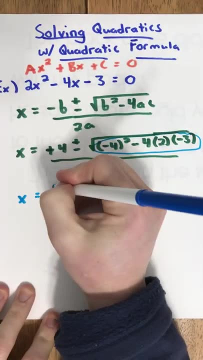 parentheses around that negative 4.. If you don't, you're going to end up with a different answer. that's going to lead you to the incorrect answer. So if you don't, you're going to end up with a different answer at the end. So we're going to do this correctly. We're going to have x equals 4,. 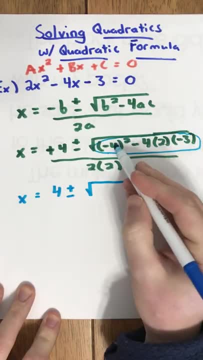 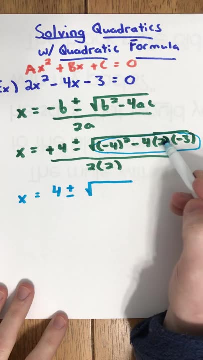 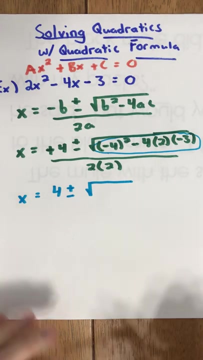 plus or minus the square root. Negative 4 squared is going to be 16.. And then negative 4 times 2 is negative 8, times a negative 3 is positive 24.. So we're going to have 16 plus 24, which is going to lead me at 40.. 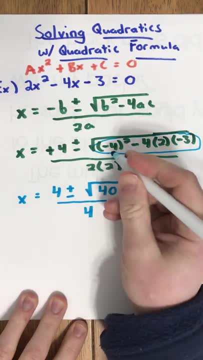 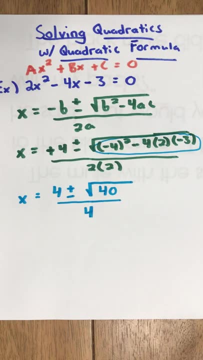 And we're going to divide this here by 4.. Alright, so you're probably going to notice that the last few times we did this, we were able to figure out what was inside that square root. We'd have a perfect square, like square root of 16, or square root of 25, where we could just pull the answer. 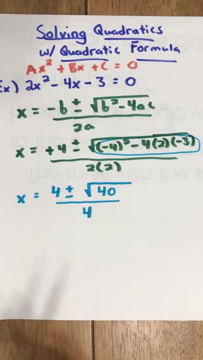 right out. In this case, we don't. So that's why we did that unit a couple days ago, where we simplified the square root of 16.. So we're going to have a perfect square like square root of 16,. 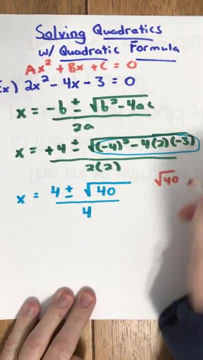 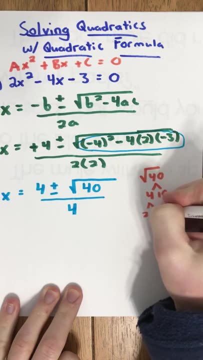 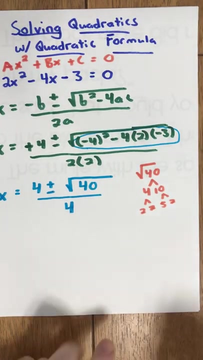 or square root of things like 40.. So off to the side here I'm going to take a look at square root of 40. And we're going to sort of factor that. So that's 4 and 10,, 2 and 2, 5 and 2.. And so I've got. 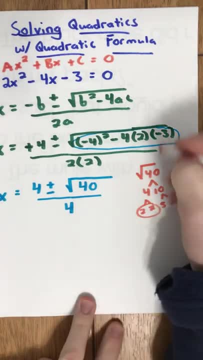 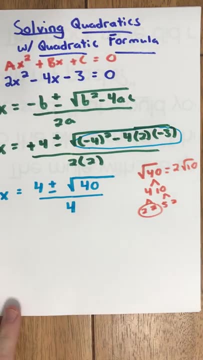 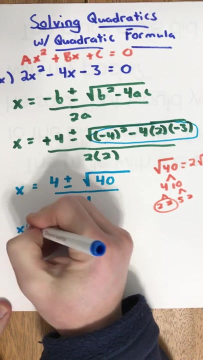 a pair of 2s that can come out. 5 and 2 are going to be inside, So the square root of 40 is the same thing as 2 squared And the square root of 10.. So what I'm going to be left with here is I'm going to have x equals 4. 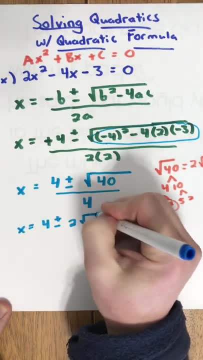 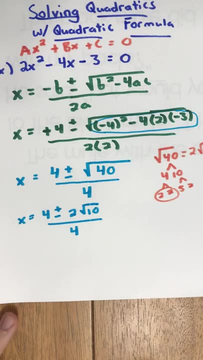 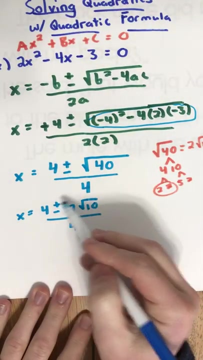 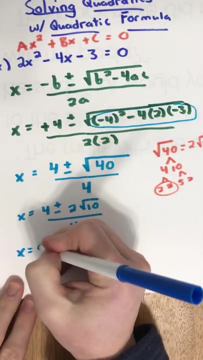 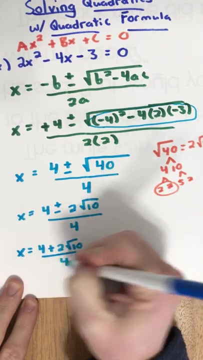 plus or minus 2 square root of 10 divided by 4.. Alright, so a little bit trickier. We've got to do our plus and we've got to do our minus. Alright, so we're going to have one answer, as x equals 4 plus 2 square root of 10 divided by 4.. And one answer. 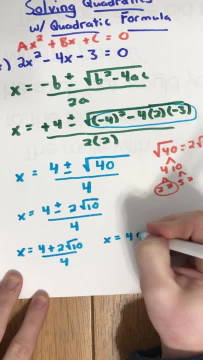 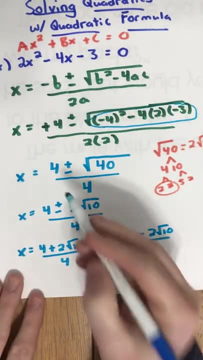 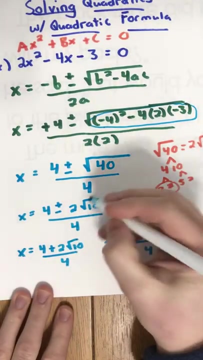 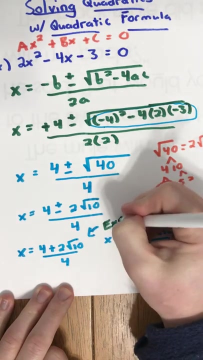 is x equals 4 minus 2 square root of 10 divided by 4.. Alright, now, the way that I have them right now, you could generally leave them like that. That is called the exact value. Okay, so this right here. put this in a different color, so it stands out. This form, this is what we.